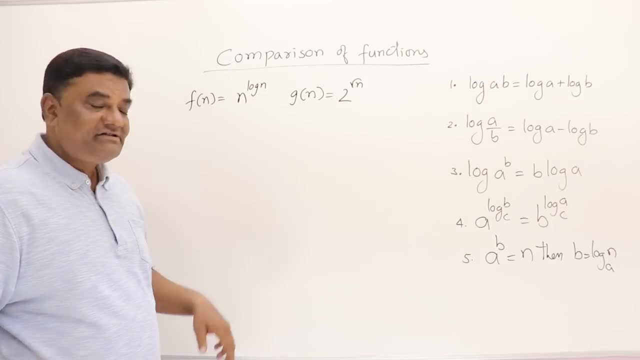 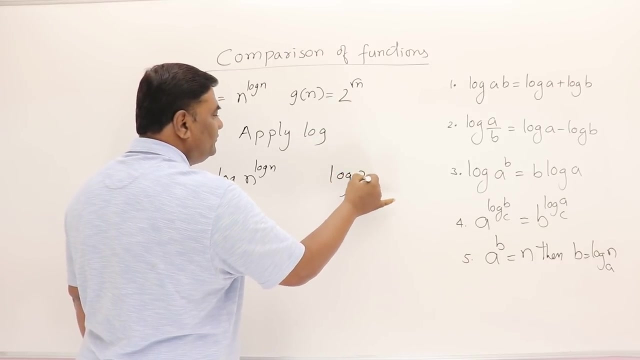 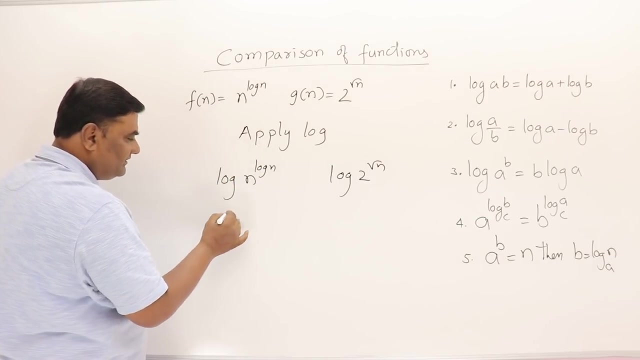 Now these two functions. Let us compare which one is greater. So for this I will apply log on both sides. So this is log of n power log n and this is log of 2 power root n. Now this power comes out by applying third formula. So this becomes log n into log n, So that power came this side. So 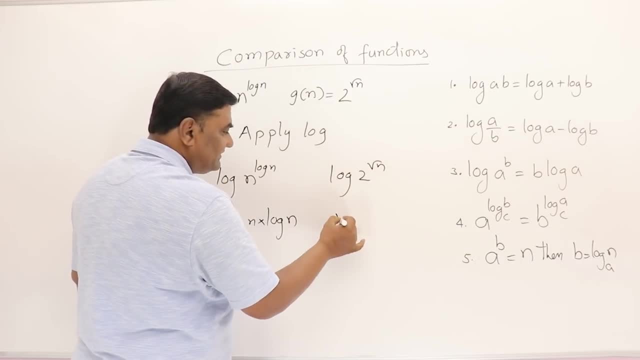 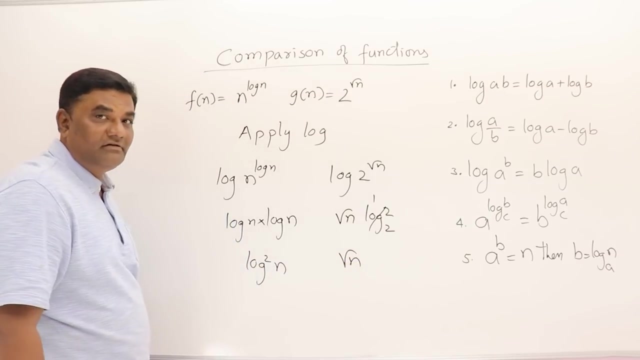 So that is log n, and now that is log n, and this power comes this side. so root n, log 2, base 2.. This is 1. now what is this? log square n and this is root n. now which one is greater? If you are unable to judge it, still, you can apply log directly. I will write the answer. 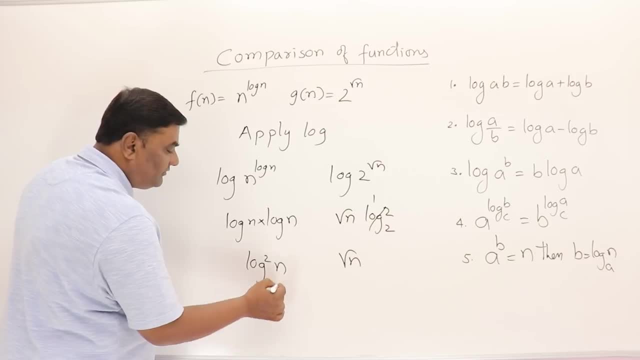 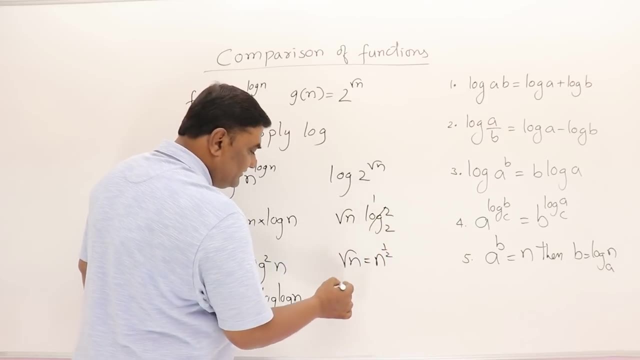 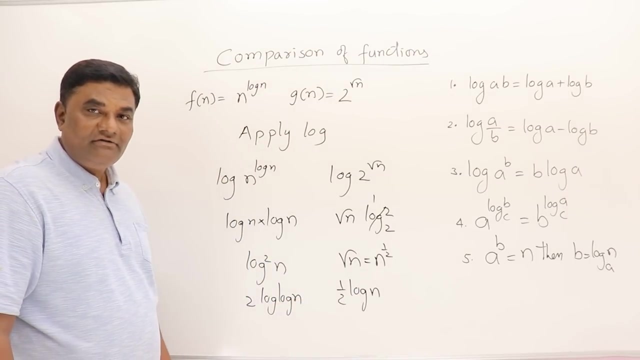 if I apply log, then this will become 2 log of log n and this becomes: this is n power 1 by 2, right, so 1 by 2 log n. Now tell me which one is smaller. log of log n is smaller than log n. yes, this is smaller. 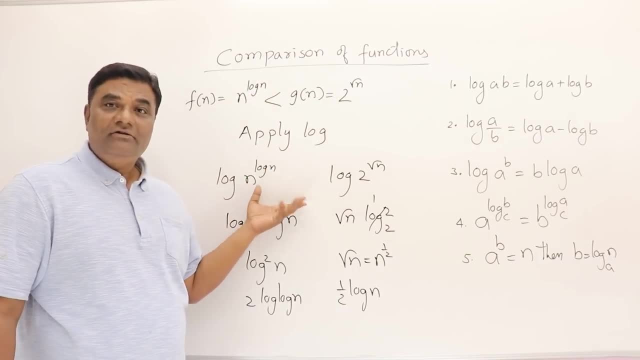 than that one With applying log for one time. if you are unable to judge it, Then you can apply log again and you can judge it. So here the thing is, we have to judge which one is smaller, which one is greater. So, for making it easy, we are applying log. there is no rule, there is no formula, right? 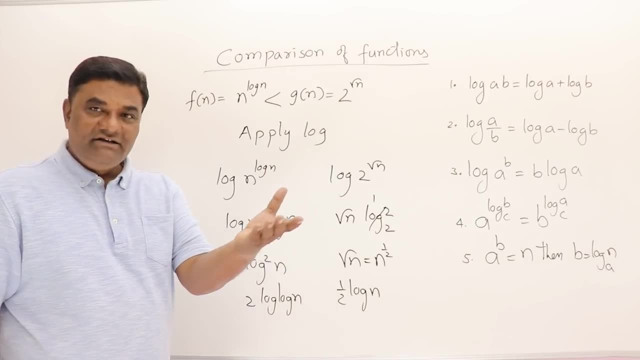 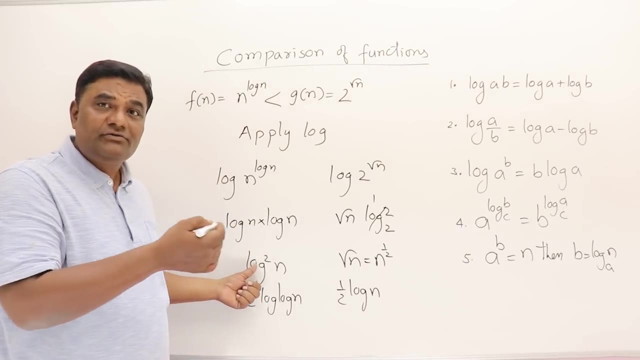 Just apply logs so that you can reduce it and see and you can easily compare them. So here we, one time applying. we were unable to do it, so we did it again. again confusion is there? log square n may be greater than just root n, because this is square, so just. 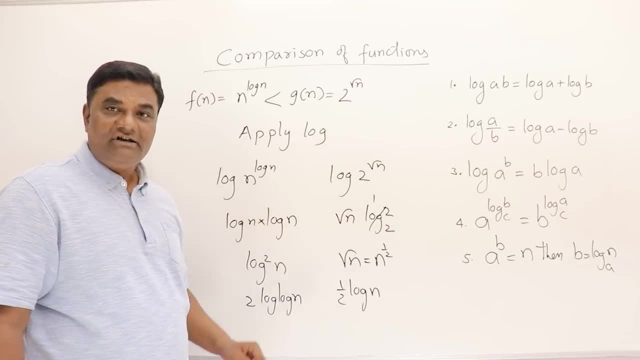 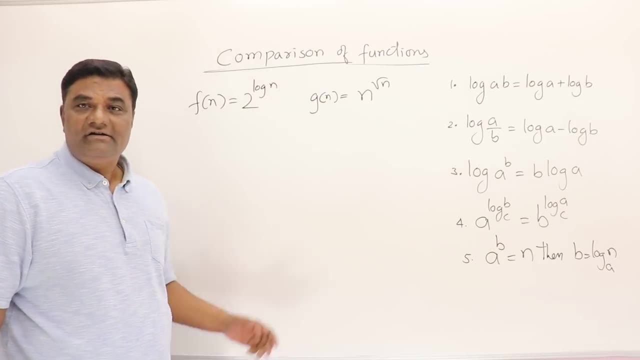 apply log one more time. So you got log of log n And that is just one log n. so log n is greater than log of log n. Now let us see who is greater. two functions apply log log n into log of 2 by 2. this is: 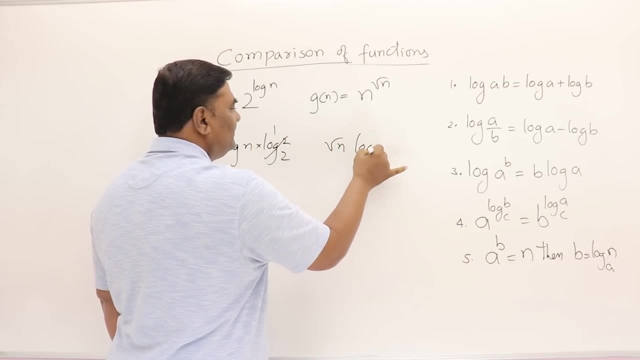 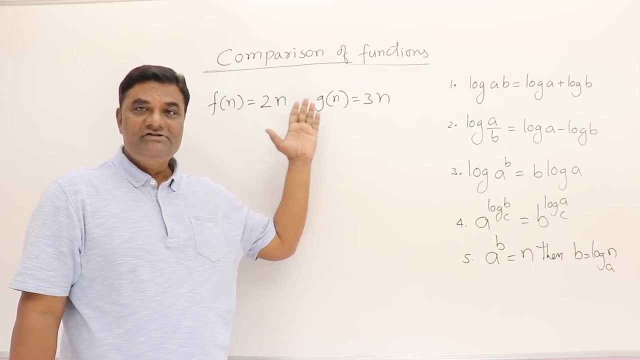 1 and this is root n log n. So what is the answer here? just log n and this is root n log n. this is greater, so this is smaller. F of n is 2n. g of n is 3n, which is smaller, which is greater. both are equal. both are equal. 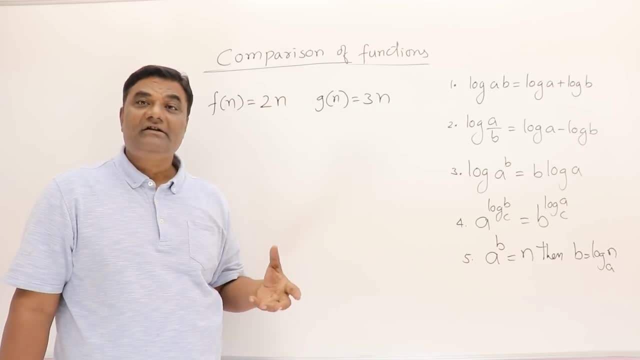 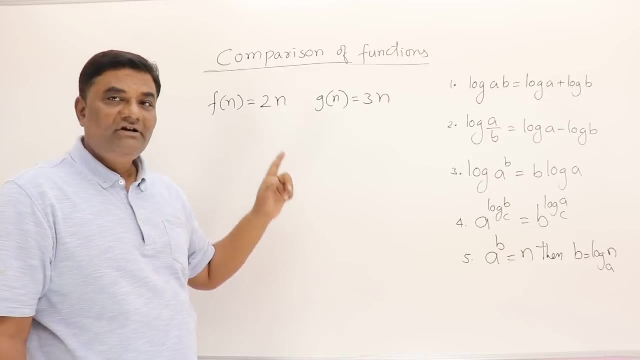 this. 2 is ignorable. 3 is ignorable when you take it asymptotically: big O of n, big O of n, or theta of n or theta of n. both are same, both are equal. both these functions are equal. Now, which function is greater? this looks smaller. this looks greater. 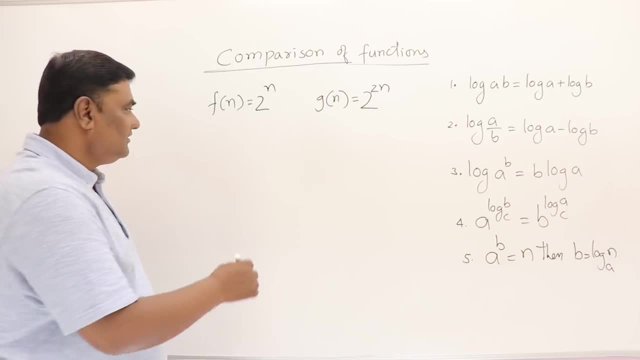 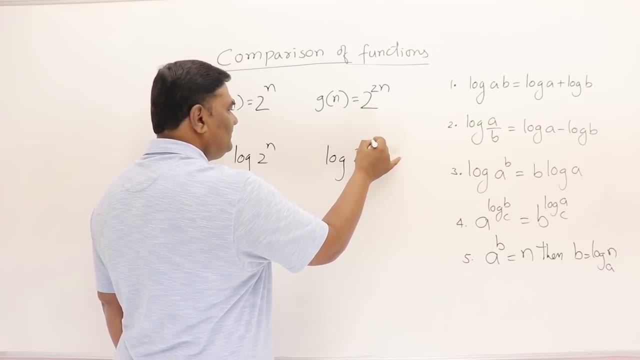 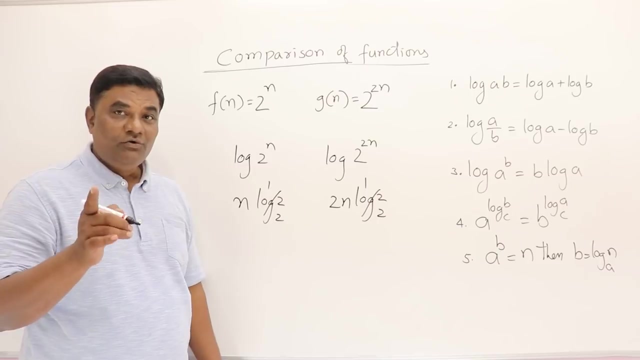 Let us apply: log of log n, This is greater, This is greater. Let us say: log log 2, power n. log 2, power 2n. so this n comes this side. log 2 by 2: this is 1, and 2n comes this side. log 2 by 2, this is 1, now, which is greater. now don't say they. 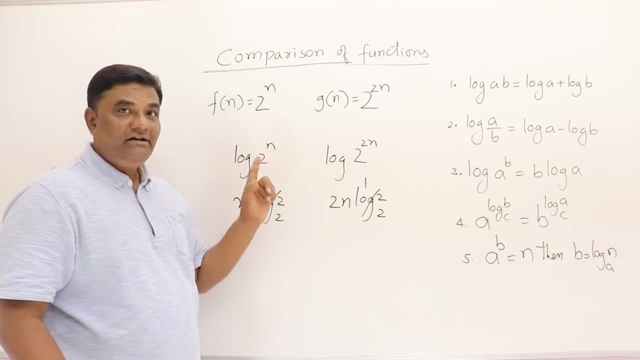 are equal. don't say, they are equal. we have applied log, then we are comparing them. now. I cannot say: ignore that too directly in the functions. you can do that now for comparison purpose. we already apply log, so you cannot strike away the coefficient. so this is 2n. 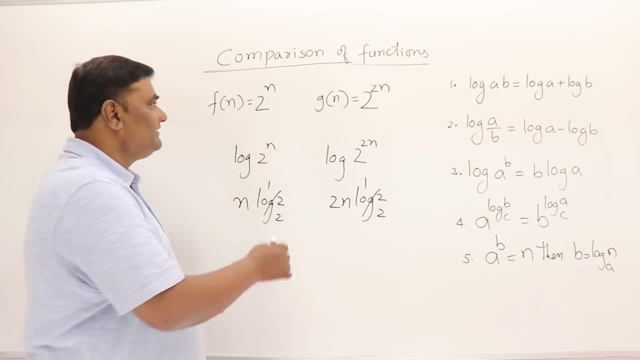 that is greater and this is smaller. so, yes, this function is smaller, that function is greater. you can clearly see from here only now. I have taken this example to make you understand: after applying log, don't cut off coefficients, don't cut off them, right in my case. I have taken this example to make you understand: after applying log, don't cut off. 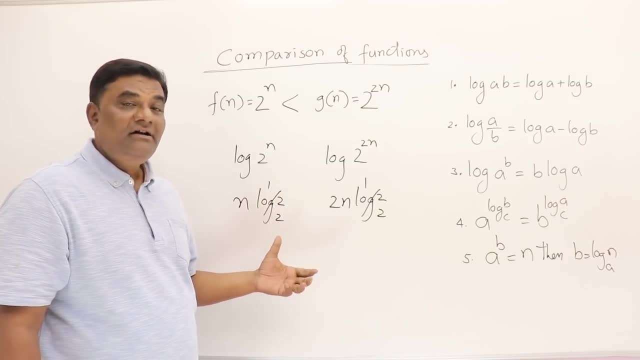 coefficients, don't cut off them. Right In one of the example I did that, but that time I did not apply log. now, after applying log, I have changed the functions. now if I cut off coefficient, it will be different answer. it will be wrong answer. directly from the functions you can cut off coefficients. so 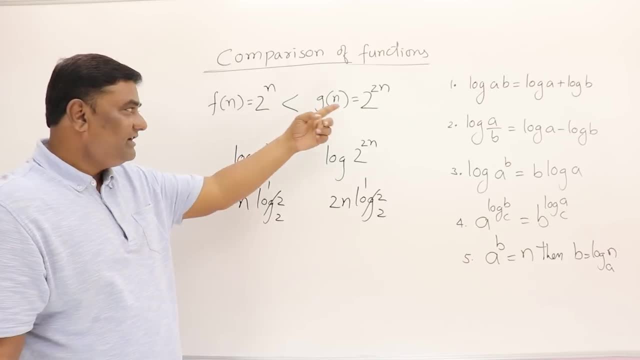 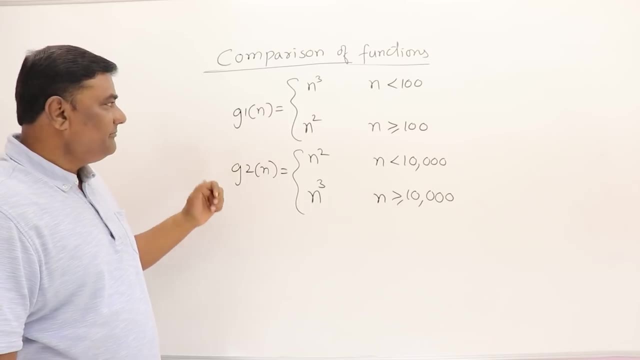 applying log. this 2n is greater than n, so that is greater. actually, this is 4 power n, this is 4 power n and this is greater than this one. this example: let us compare two functions, g1 and g2. which one is greater? 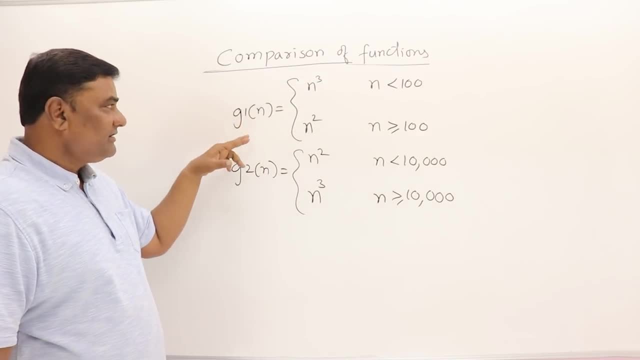 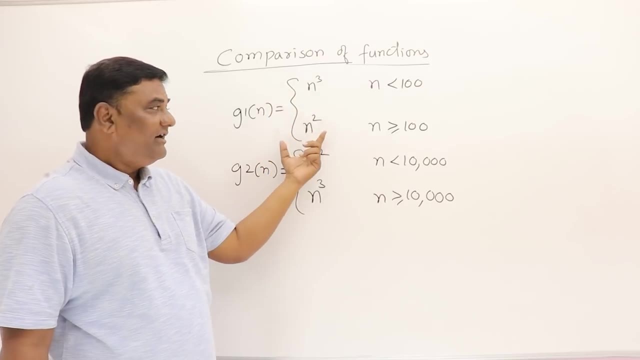 Which one is greater. Now, here it is not a single expression. here is n cube or n square. so for n value, let us say 100, it is n cube, after that it is n square. so this is reducing, and this is n square, up to 10000. after that this is n cube. if I take n values, let us say this is 100 and this is. 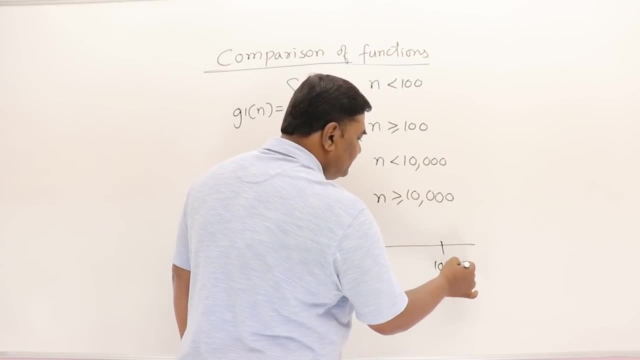 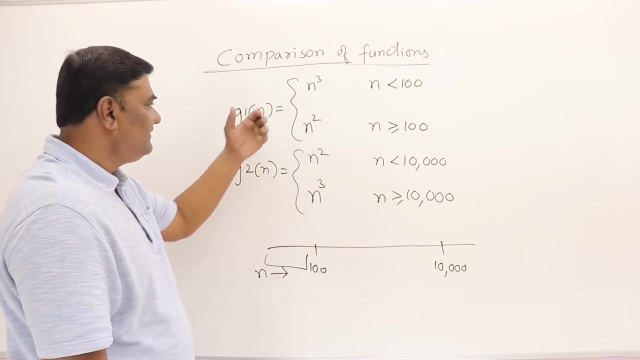 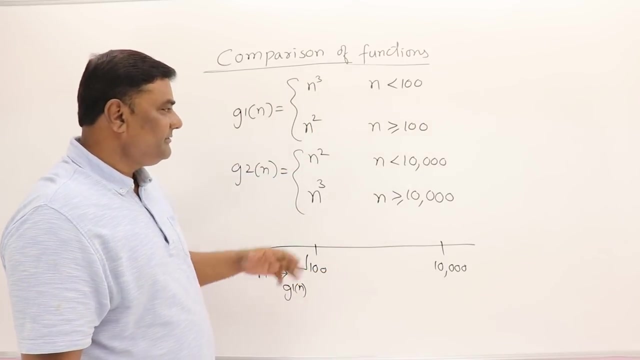 n and this is 10000.. Now, on this side, who is greater? this side, less than 100, g1 is greater, and from 100 to 10000, who is greater? because the figures are there. so I have used this on the bar now from: 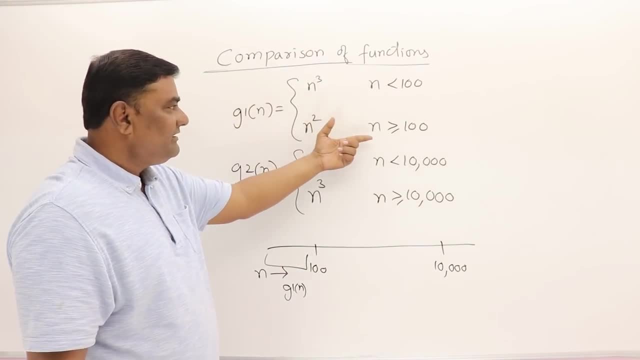 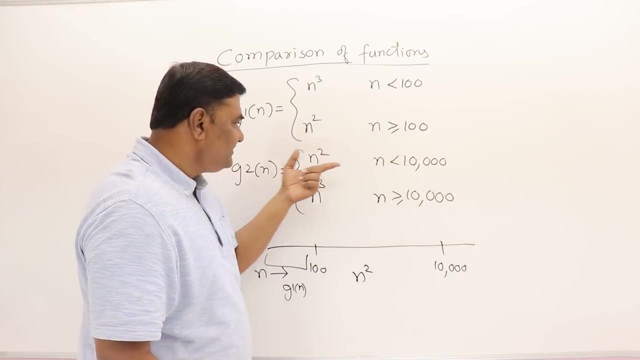 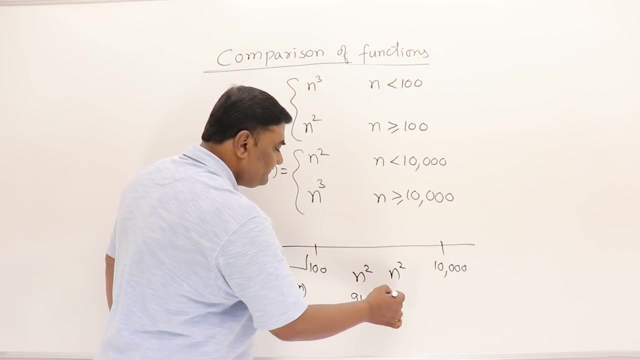 100 to 10000. who is greater? see 100 to. from 100 onwards, this is just n square, and below 10000 also. this is also n square. So this is also n square. So this is also n square. So both are n square. so g1 is equal to g2.. 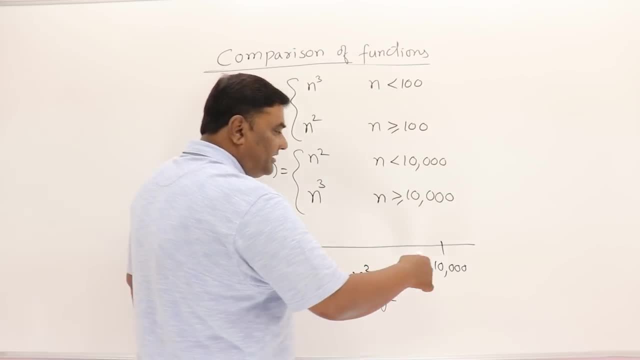 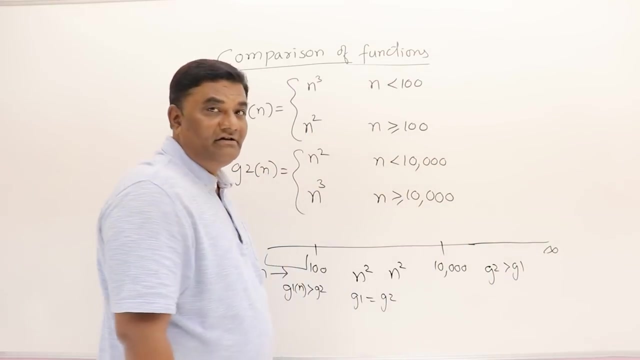 Here g1 was greater than g2, but beyond 10000, beyond 10000. so 10000 is n square, only after 10000 this is n cube. so g2 is greater than g1. so this is still where this is infinity. Now, who is greater? which function is greater, g1 or g2.. 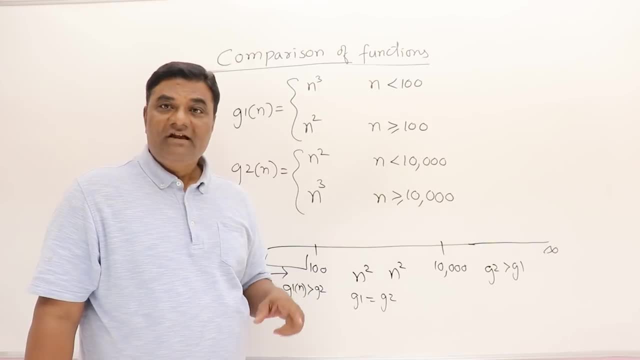 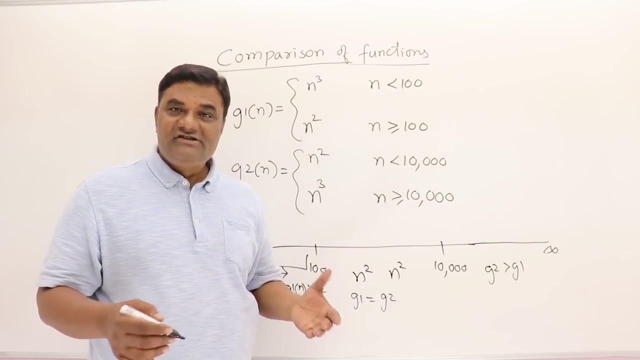 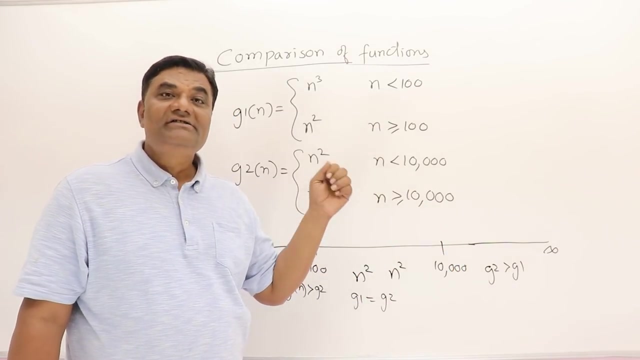 g2 is greater always. from what value? of n? from 10000 onwards, it is always greater. before 10000, they were changing their sides sometime. this was greater or they were equal. but from that point onwards, 10000 onwards, always g2 is greater. so g2 is greater than g1. g2 is greater. 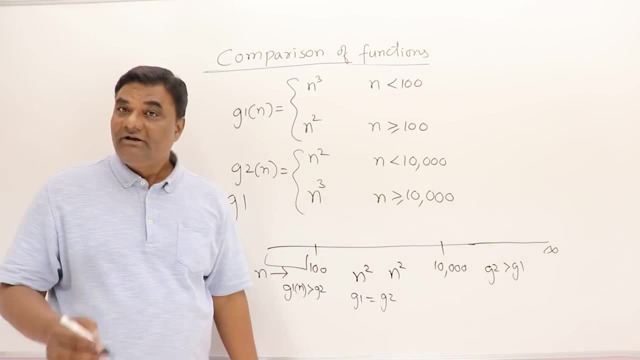 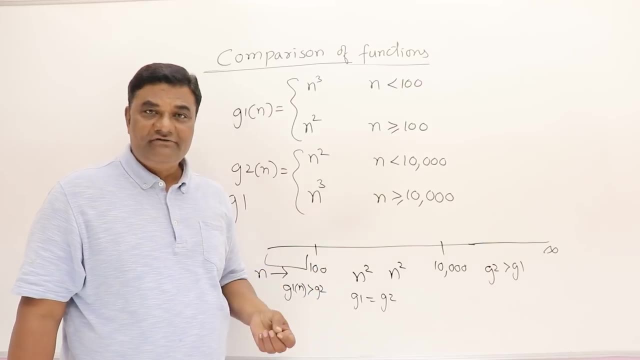 than g1. So remember this. So whenever you say some function is greater than g1. So remember this. So whenever you say some function is greater than g1. So every function is greater than other function, You don't have to take the small values of n. it can be from very large values of n also. 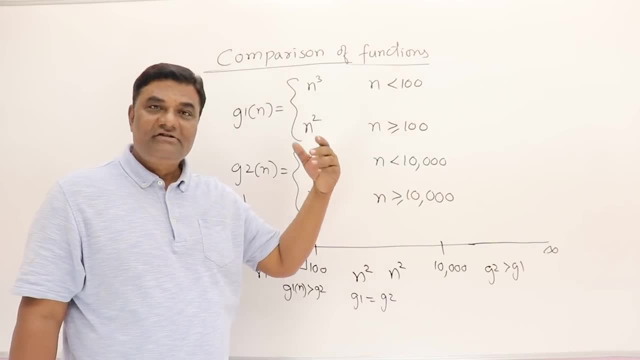 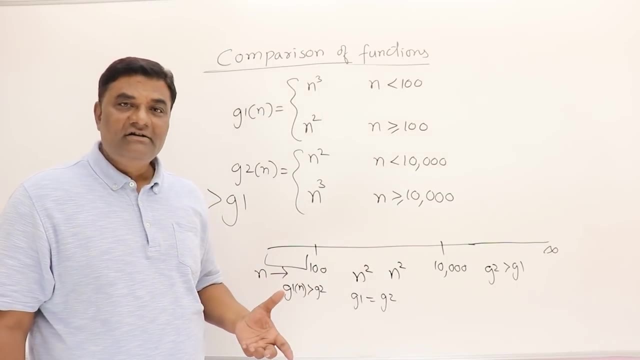 but from that point, if it is always greater than we consider that function as greater, Alright, we don't just check into smaller values and decide for all values of n. we decide means up to infinity. So from 10000 to infinity, there is no limit. there is no limit. so g2 is always greater. 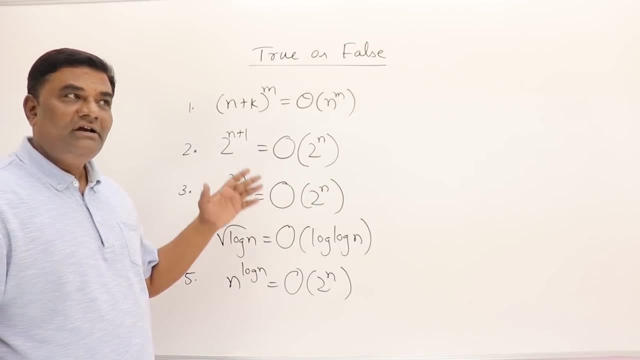 than g1.. some asymptotic notations are given and comparison is there, so we have to find out whether these statements are true or false. Let us check. this is n plus k, whole power m, and if you open this binomial right, two terms are there. so if you open this, it will be n power m. that. 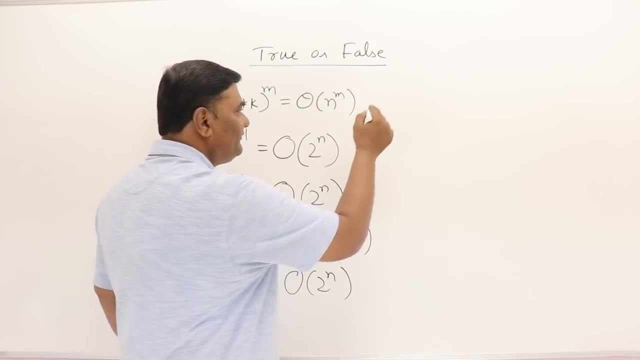 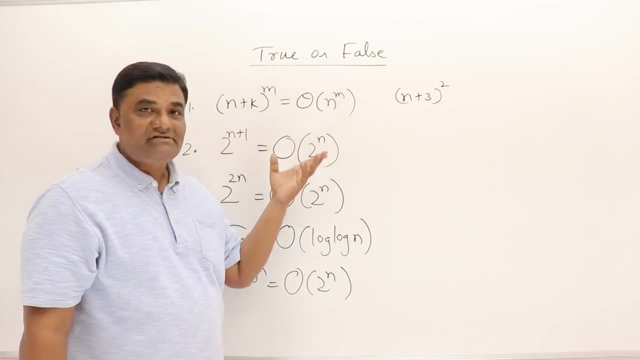 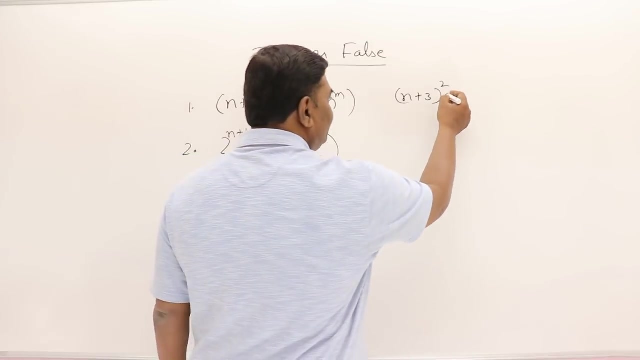 is going to be a highest term. It is just like, for example, n plus three, whole square. then what is the highest term you get there? n square is the highest term. so if m is there as a power, so n power, m is the highest term. so we can write this as theta of n? square. 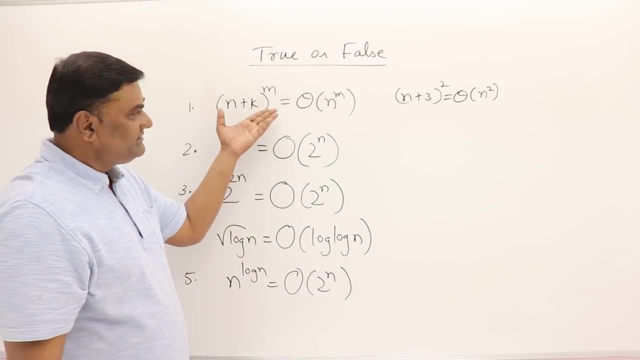 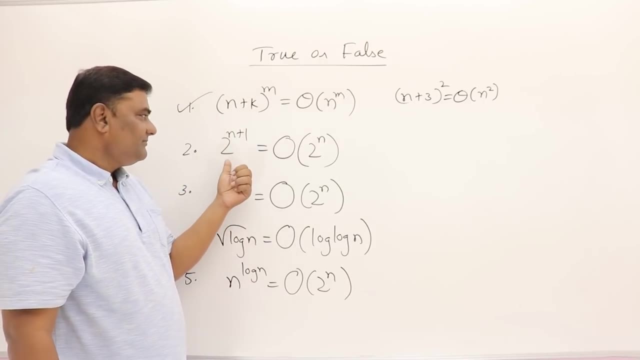 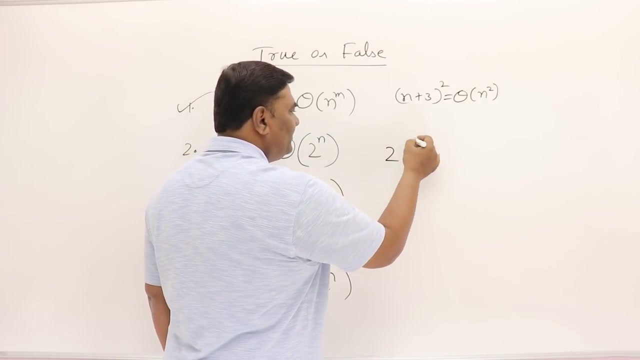 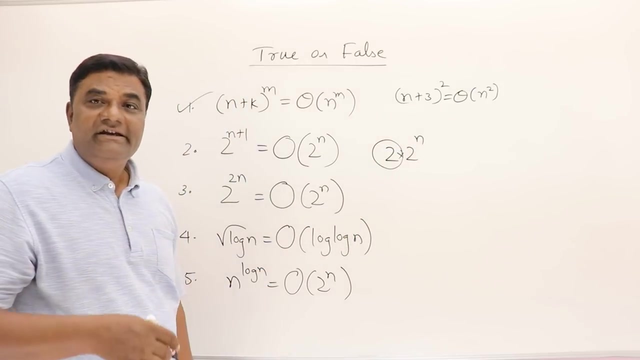 yes, it is exactly theta of n square. so this is theta of n power m. yes, correct, this is correct. Then what about this one, Two power n plus one, so this is two into two power n. 2 into 2 power n coefficient is ignorable and it is theta of 2 power n also. big O also. 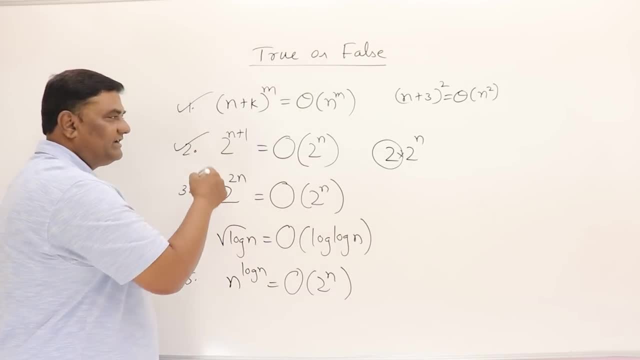 omega also anything you can write. so this is also correct, big os, correct. then let us take this one: 2 raise to 2, 2n and this is 2 raise to m. this is 4 power n and that is 2 power n. 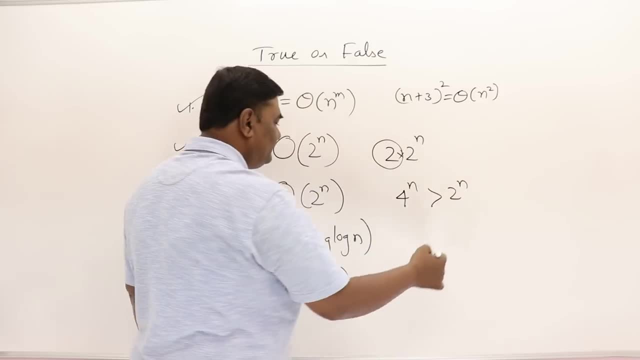 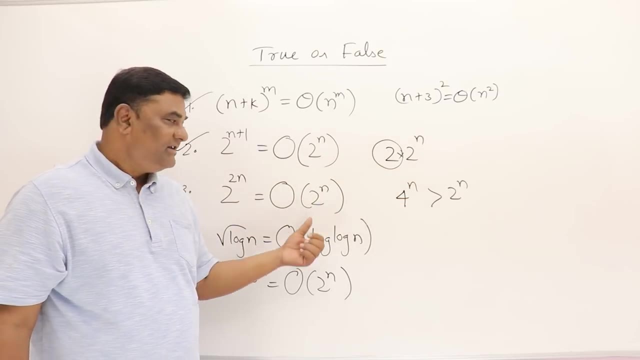 1 minus 4 power m. 2 raise to 1 is just 4 energy. 1 minus 4 power m is just 1 cost. 1 plus 1 is just 1 cost than 2 power n. 2 power n cannot be an upper bound for this one, wrong, so it. 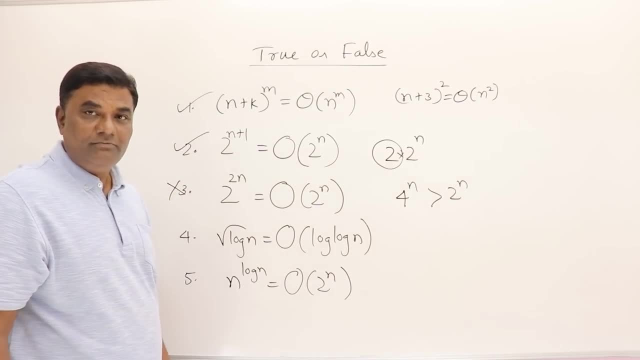 should be big of 4 power n, not 2 power n. this is wrong. the next, this one: this is root of log n. this is log of log n. which one is greater? you apply log on both side and check it. if you apply log, you get what? 1 by 2 log of log n there.